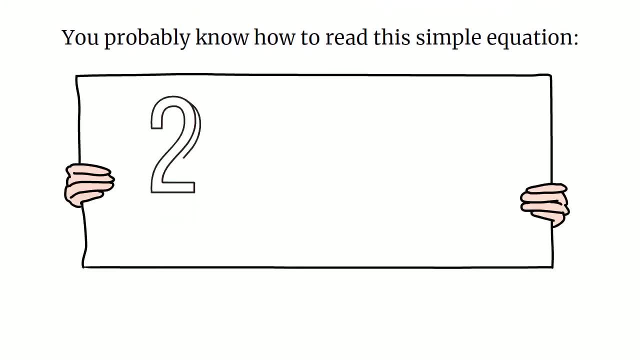 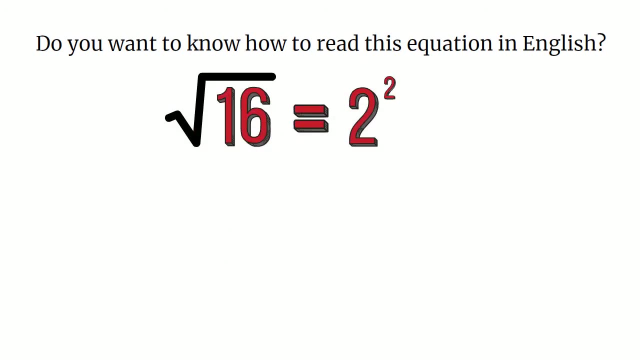 You probably know how to read this simple equation: It's 2 plus 2 equals 4.. However, do you want to know how to read this equation in English Or this? If you do, then this video is for you. Please note that this is not a maths lesson. 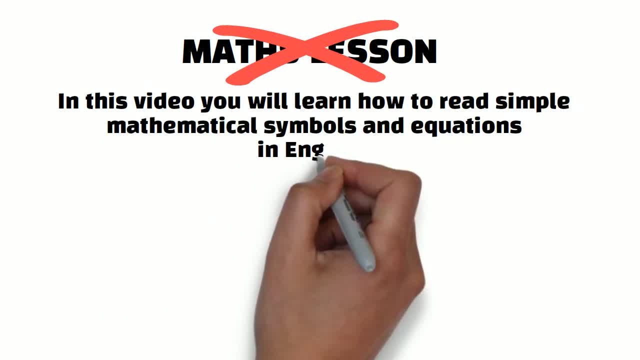 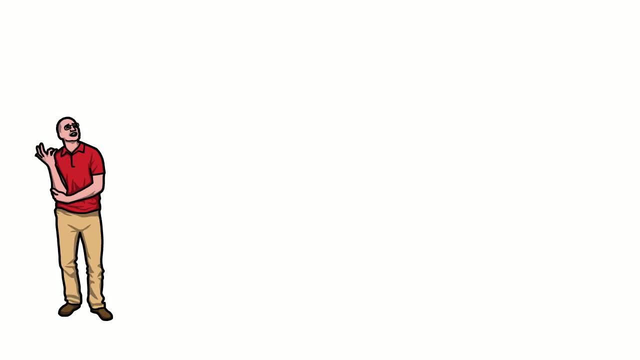 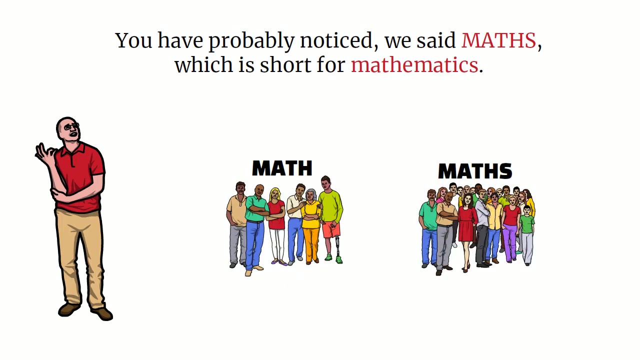 In this video, you will learn how to read simple mathematical symbols and equations in English. Before we start, we would like to explain something that you have probably noticed. We said maths as a short form for mathematics. You may wonder why other people say math as opposed to maths. 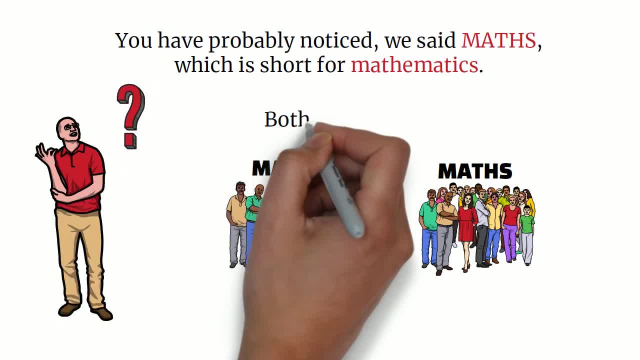 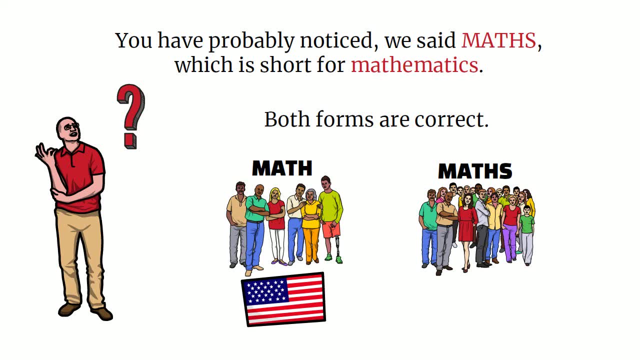 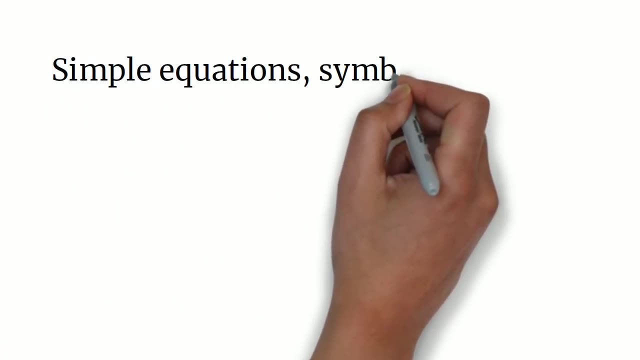 And you don't know which one is correct. Be assured, Both forms are correct. However, math is more common in American English and maths is used in British English. Okay, so let's go. We'll start with simple equations and symbols first, and basic mathematical operations. 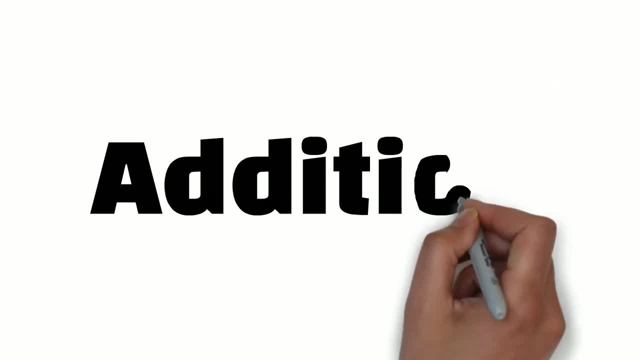 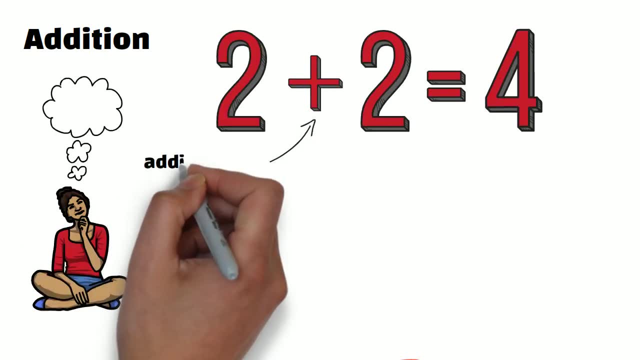 First addition. You will probably know this one. The symbols here are like this. There are the addition sign, or the plus sign, and the equal sign, Sometimes also called the equal sign without the s at the end. The result or the total of an addition equation is called a sum. 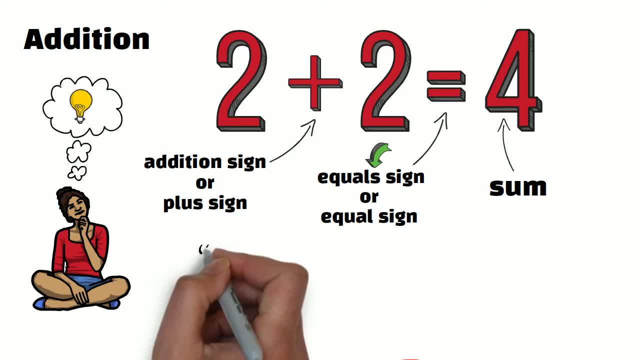 We read the whole equation like this: 2 plus 2 equals 4.. Or you could say: 2 and 2 is 4.. Or if you want to explain this to someone, then you could say: If you add 2 and 2 together, you get 4.. 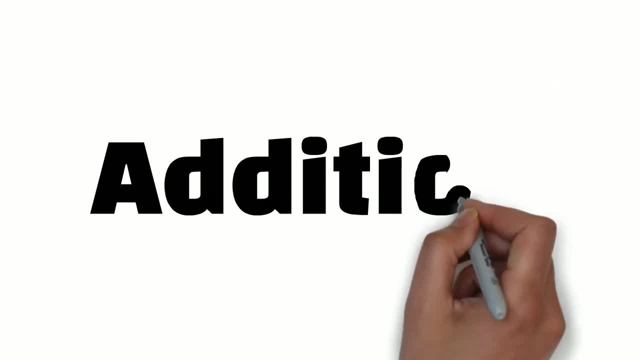 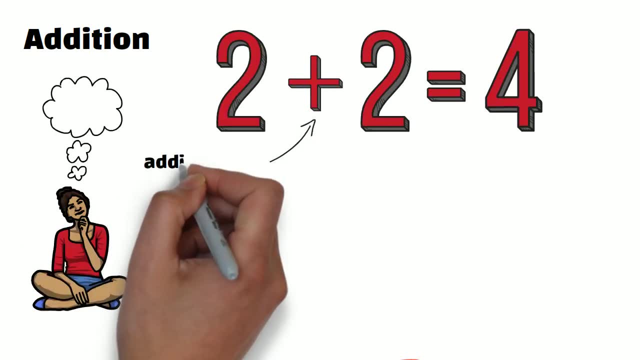 First addition. You will probably know this one. The symbols here are like this. There are the addition sign, or the plus sign, and the equal sign, Sometimes also called the equal sign without the s at the end. The result or the total of an addition equation is called a sum. 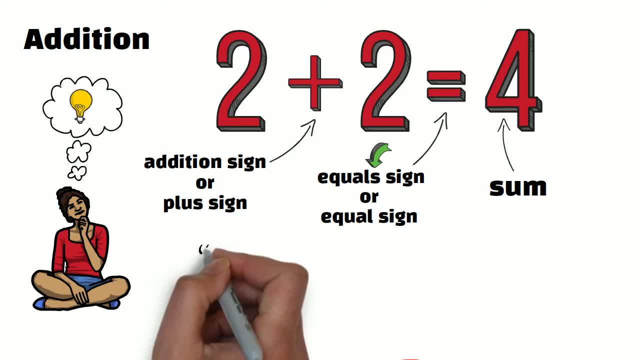 We read the whole equation like this: 2 plus 2 equals 4.. Or you could say: 2 and 2 is 4.. Or if you want to explain this to someone, then you could say: If you add 2 and 2 together, you get 4.. 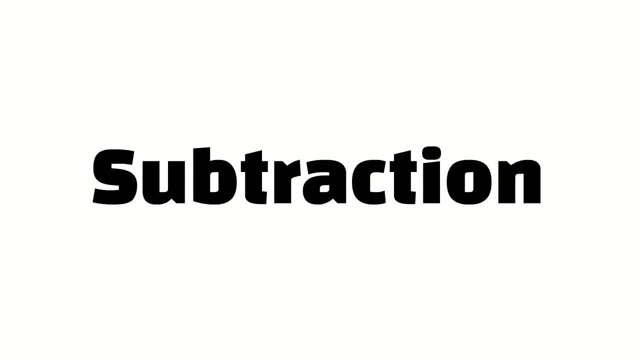 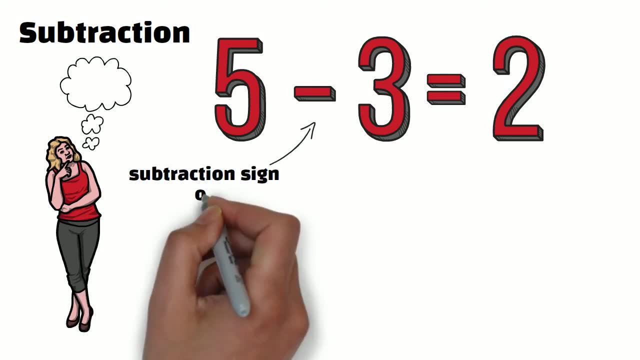 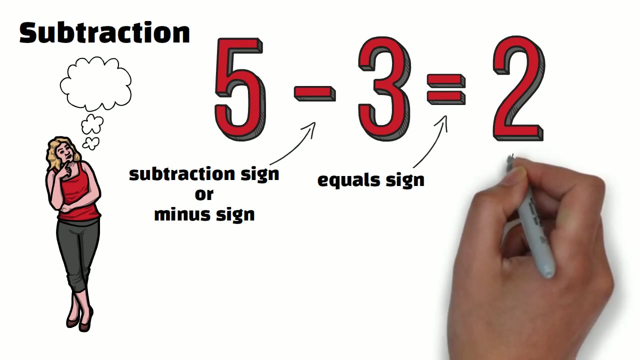 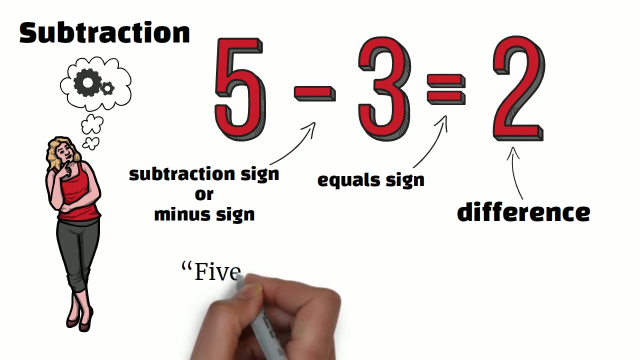 Let's now move on to subtraction. The symbols used here are the subtraction sign or the minus sign And again the equals sign. The result of a subtraction equation is called a difference. We read the whole equation like this: 5 minus 3 equals 2.. 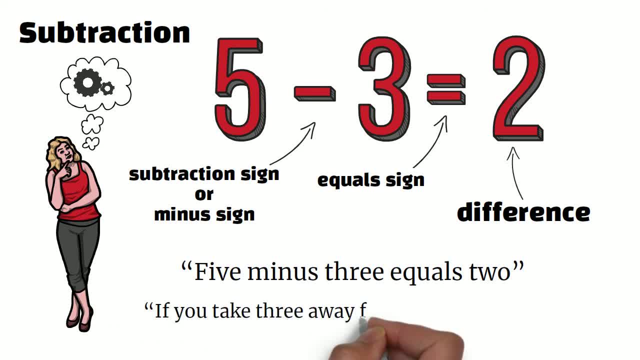 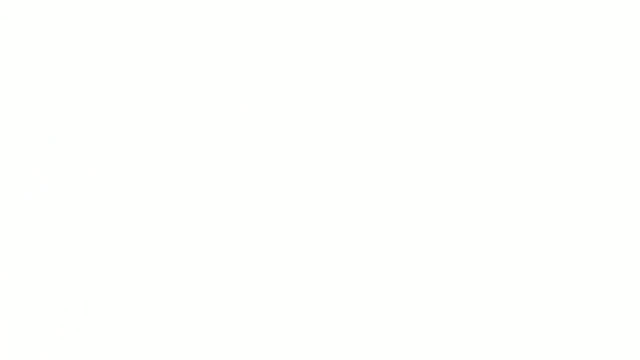 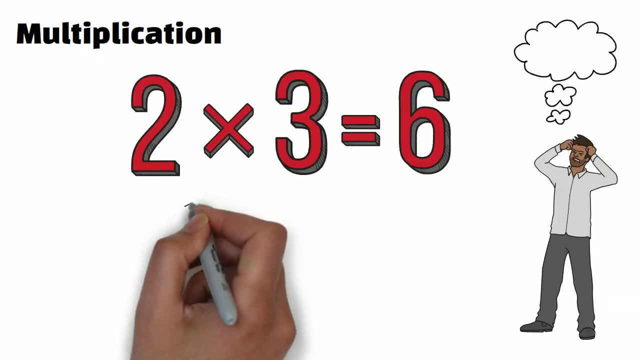 Or if you wanted to explain this to someone, you could say: If you take 3 away from 5, you get 2.. Okay, Let's now move on to subtraction. Let's now move on to multiplication. The symbols used here are the multiplication sign or the times sign. 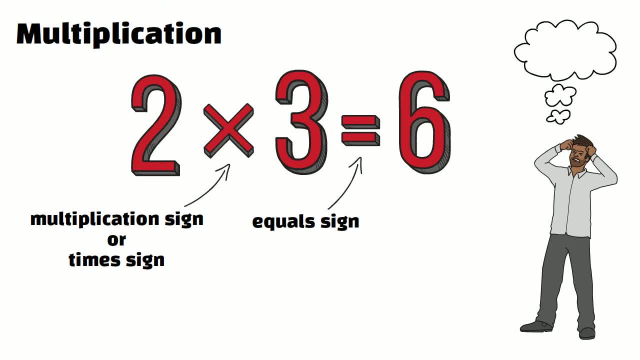 And again the equals sign. The result of a multiplication equation is called a product. We read the whole equation like this: 2 times 3 equals 6.. or if you wanted to explain this to someone, you could say: if you multiply 2: 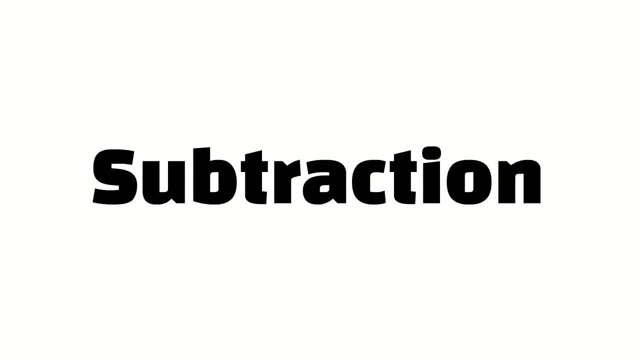 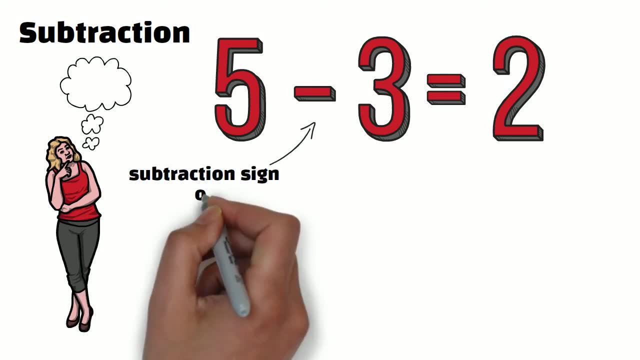 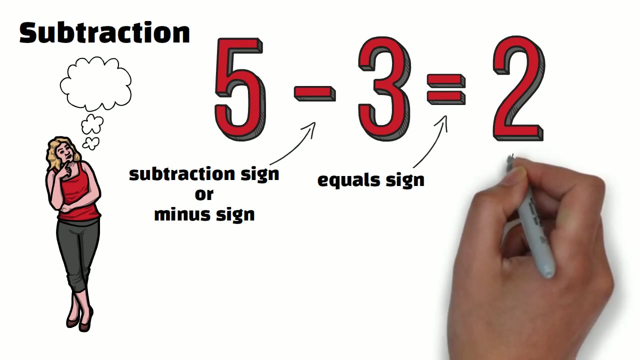 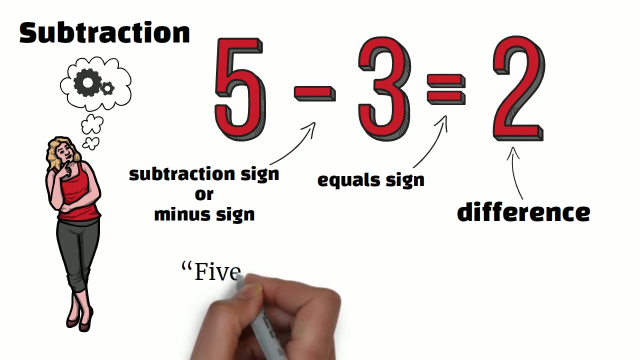 Let's now move on to subtraction. The symbols used here are the subtraction sign or the minus sign And again the equals sign. The result of a subtraction equation is called a difference. We read the whole equation like this: 5 minus 3 equals 2.. 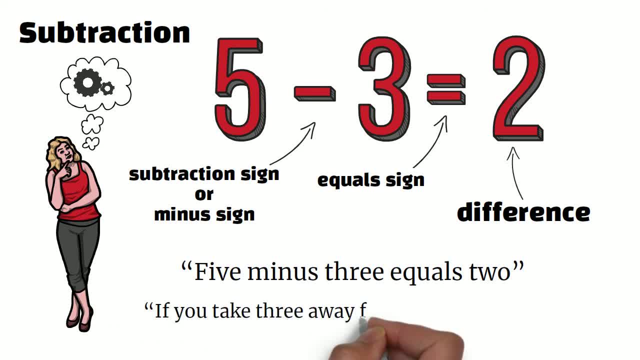 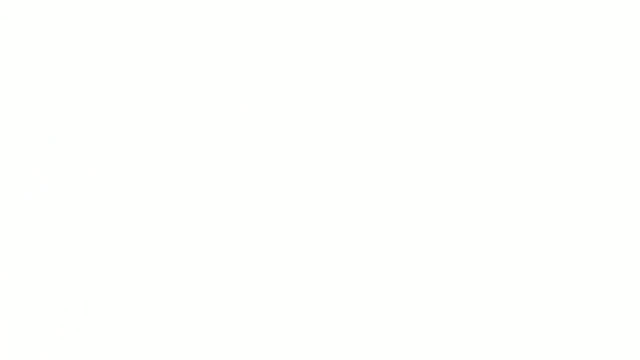 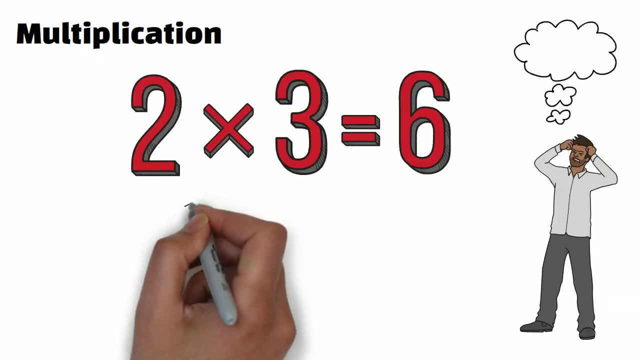 Or if you wanted to explain this to someone, you could say: If you take 3 away from 5, you get 2.. Okay, Let's now move on to subtraction. Let's move on to multiplication. The symbols used here are the multiplication sign or the times sign. 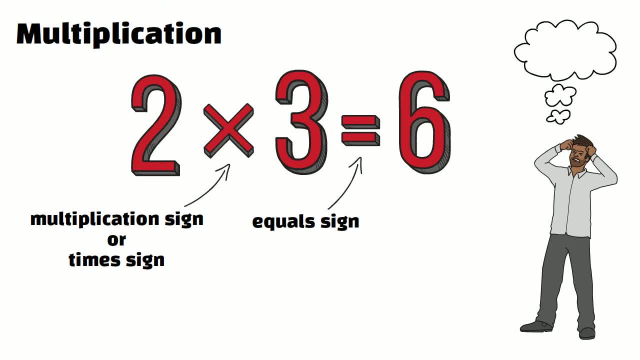 And again the equals sign. The result of a multiplication equation is called a product. We read the whole equation like this: 2 times 3 equals 6.. or if you wanted to explain this to someone, you could say: if you multiply 2: 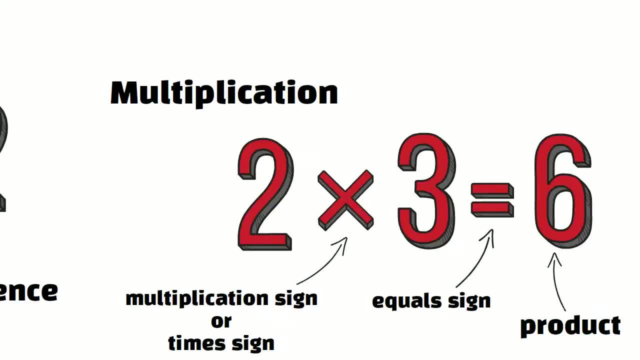 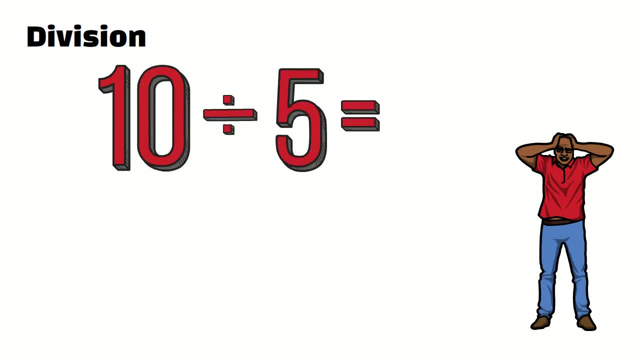 by 3, you get 6. let's now move on to division. the symbols used here are the division sign and again the equal sign. the result of a division is called a quotient. we read the whole equation like this: 10 divided by 5 equals 2, or if. 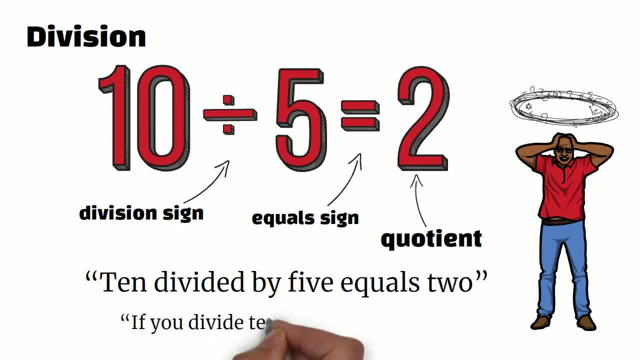 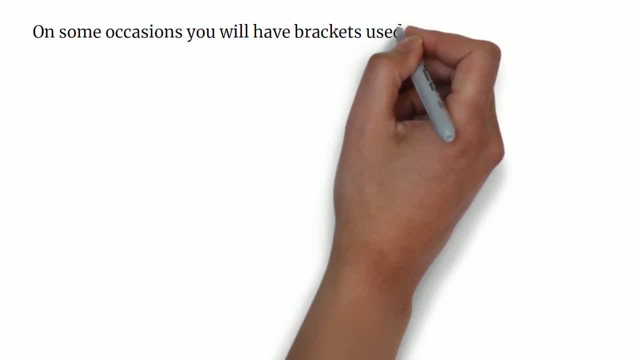 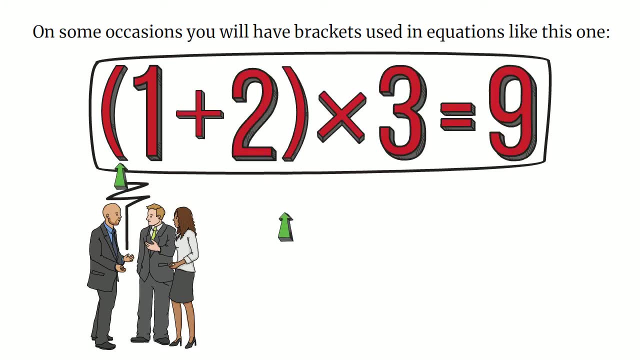 you wanted to explain this to someone, you could say: if you divide 10 by 5, you get 2. it is also worth mentioning that on some occasions, you will have brackets used in the equations like this one. we read this as one plus two. in brackets, times three equals nine. Okay, we have now covered the. 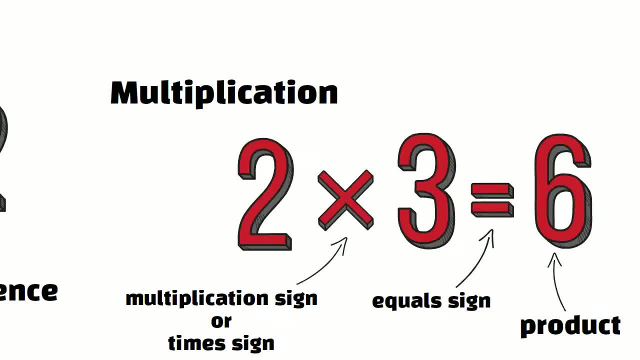 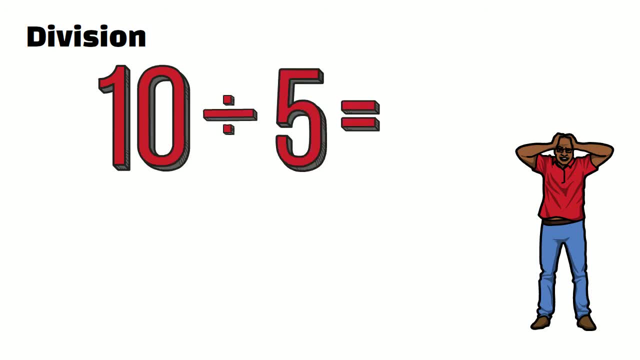 by 3, you get 6. let's now move on to division. the symbols used here are the division sign and again the equal sign. the result of a division is called a quotient. we read the whole equation like this: 10 divided by 5 equals 2, or if you. 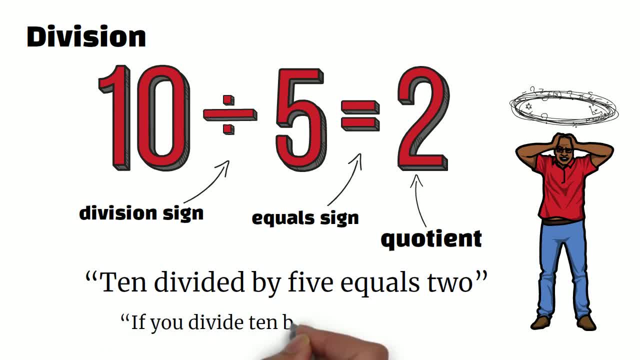 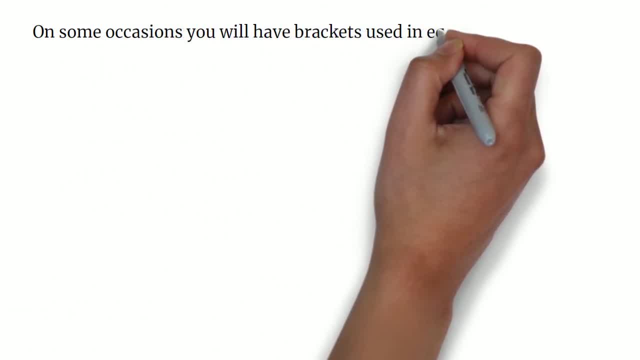 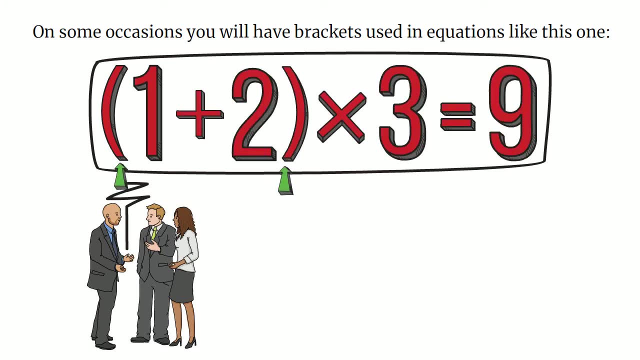 wanted to explain this to someone. you could say: if you divide 10 by 5, you get 2. it is also worth mentioning that on some occasions you will have brackets used in the equations like this one. we read this as one plus two. in brackets, times three equals nine. Okay, we have now covered the 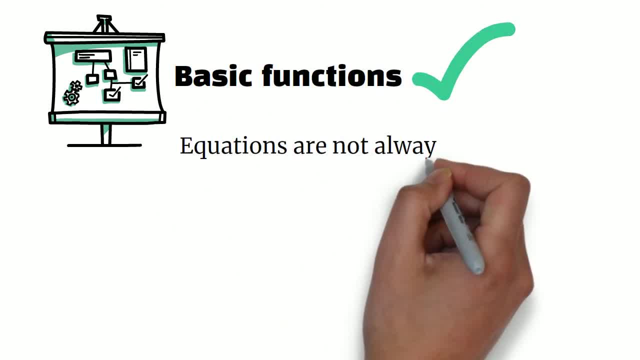 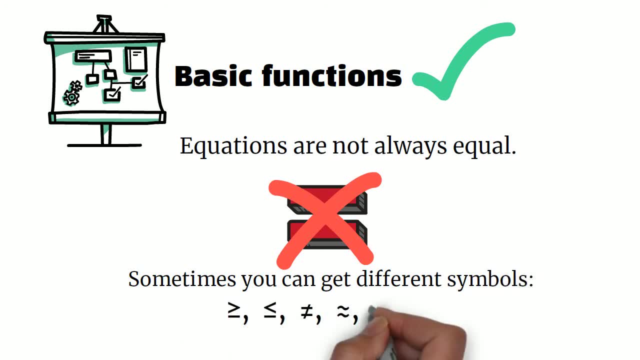 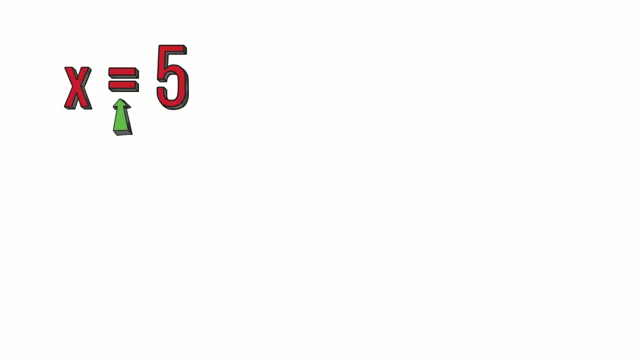 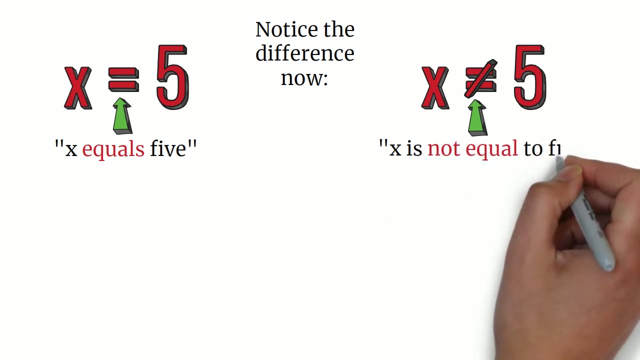 basic functions. As you know, equations are not always equal. Sometimes you could get different symbols instead of the equals sign. Let's see some examples. We learned this one already: X equals five. But notice the difference now. This is how we read it: X is not equal to five. Or another one: X is greater than five. Or 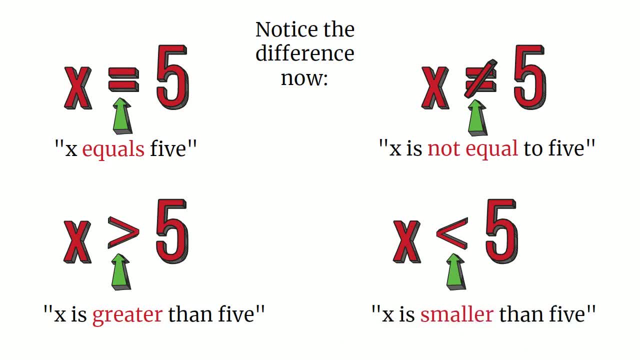 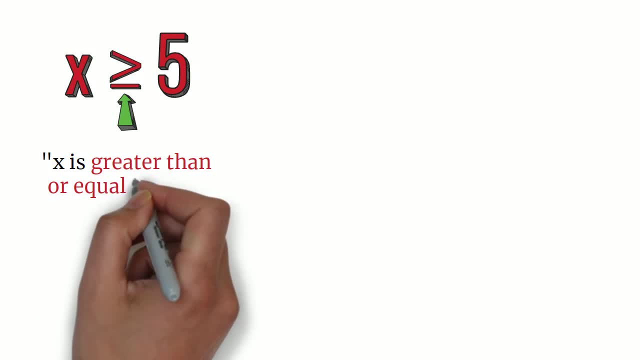 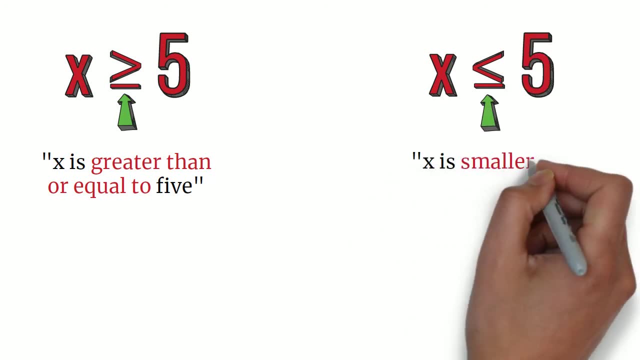 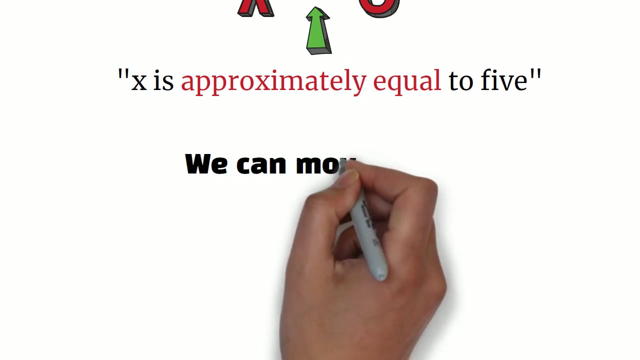 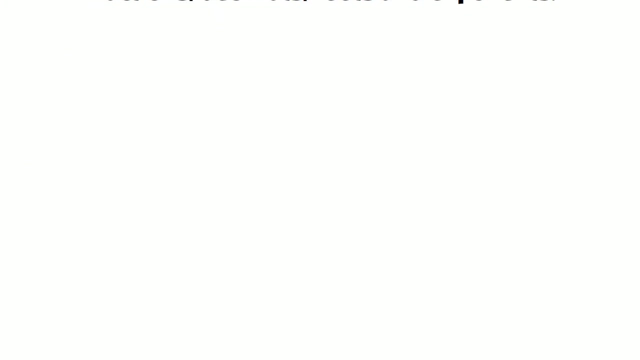 X is smaller than five. Or another example: X is greater than or equal to five. Or X is smaller than or equal to five. And one more: X is approximately equal to five. Okay, now we can move on to fractions, Decimals, roots and exponents. First fractions: The number at the top is the. 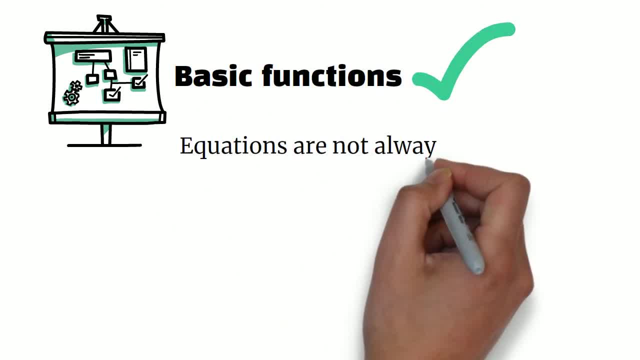 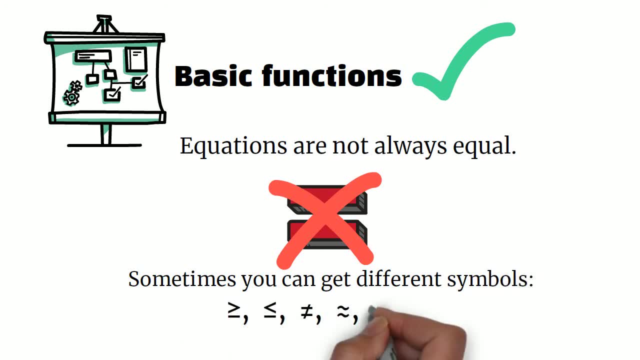 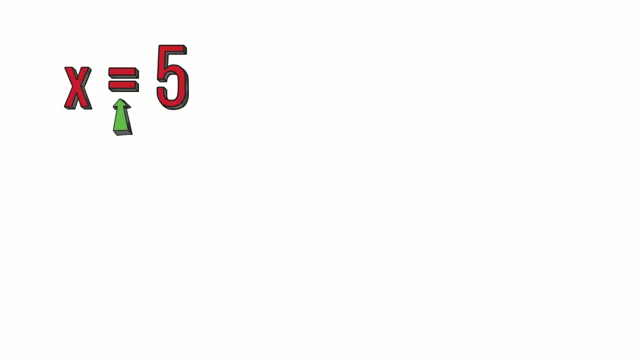 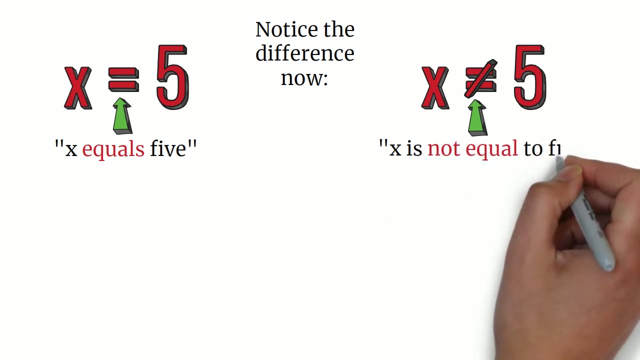 basic functions. As you know, equations are not always equal. Sometimes you could get different symbols instead of the equals sign. Let's see some examples. We learned this one already: X equals five. But notice the difference now. This is how we read it: X is not equal to five. Or another one: X is greater than five. Or 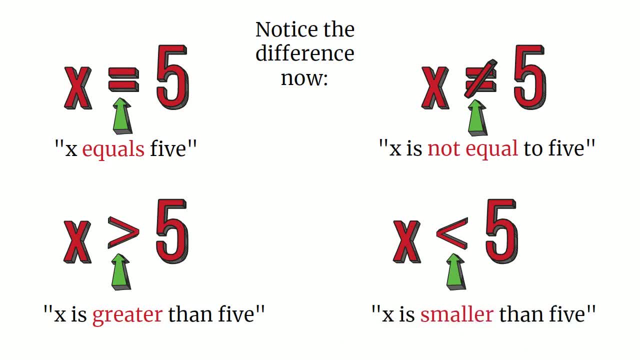 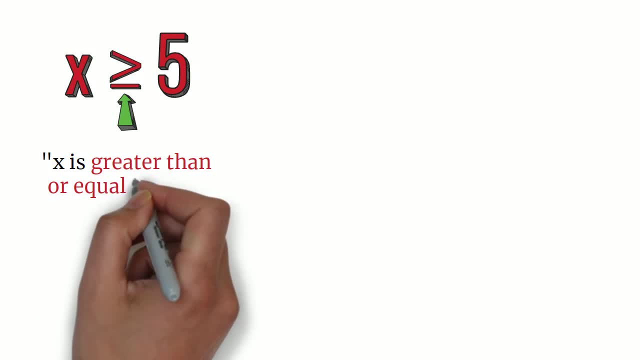 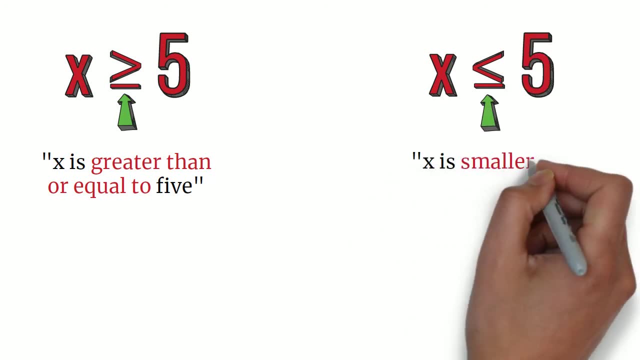 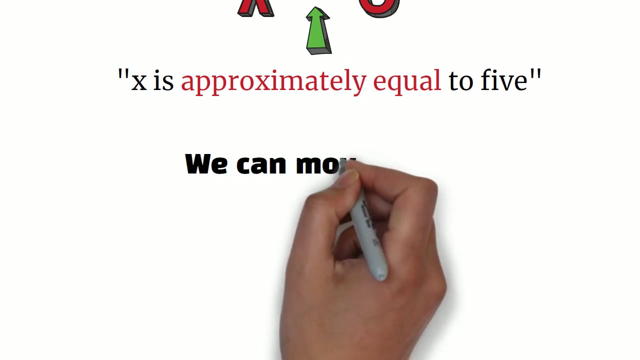 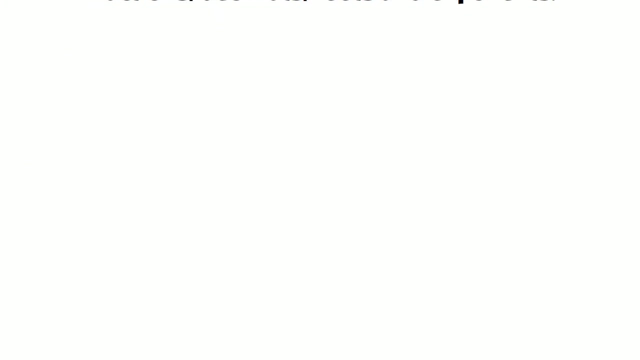 X is smaller than five. Or another example: X is greater than or equal to five. Or X is smaller than or equal to five. And one more: X is approximately equal to five. Okay, now we can move on to fractions, Decimals, roots and exponents. First fractions: The number at the top is the. 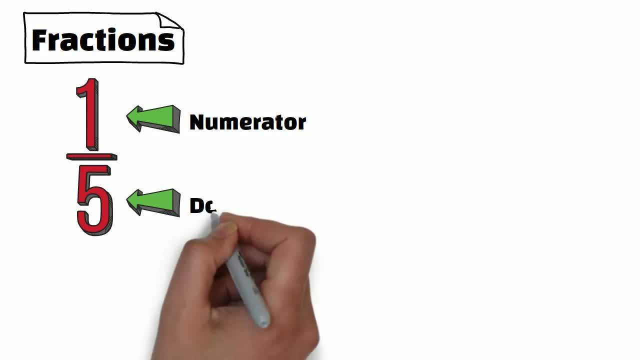 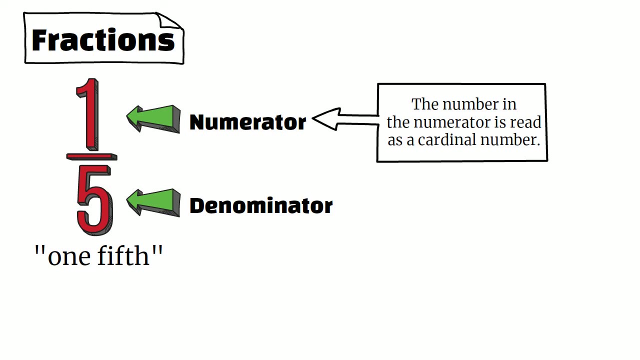 numerator And the number at the bottom is the denominator. We read this fraction as one fifth. As you can see, the number in the numerator is read as a cardinal number. The number in the denominator is read as an ordinal number. If the number in the numerator 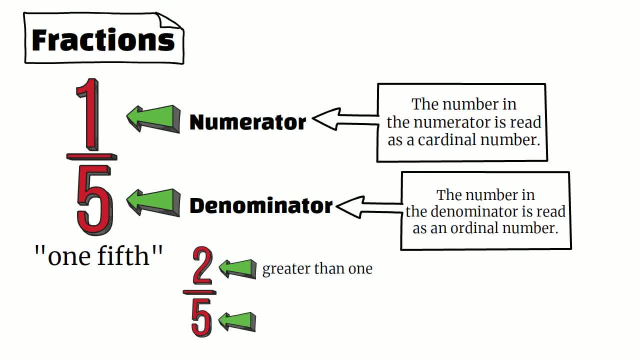 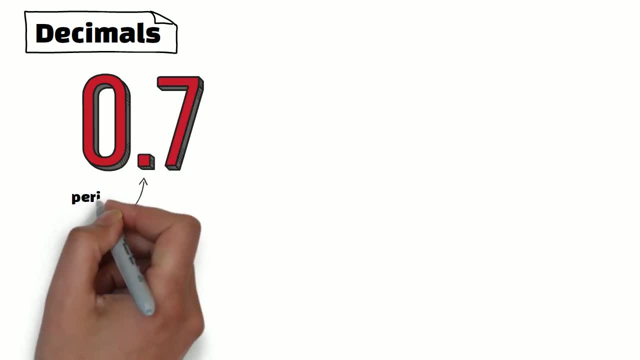 is greater than one, then we add S to the ordinal number in the denominator, For example two fifths. Let's now move on to decimals. The dot in the middle is the period or the decimal point. Let's see how we read it: Zero point seven. Or we could read it as we read fractions. 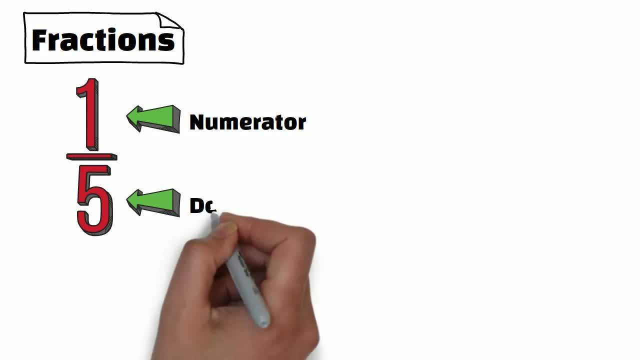 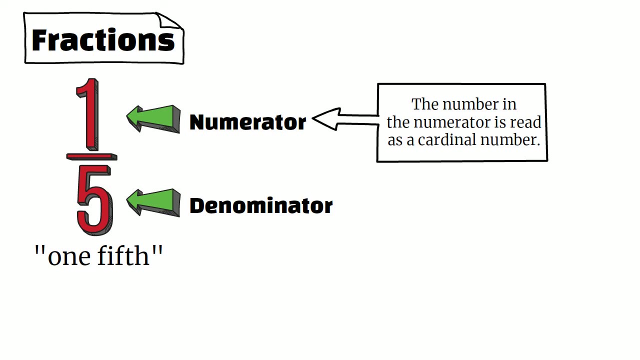 numerator and the number at the bottom is the denominator. We read this fraction as one fifth. As you can see, the number in the numerator is read as a cardinal number. The number in the denominator is read as an ordinal number. If the number in the numerator 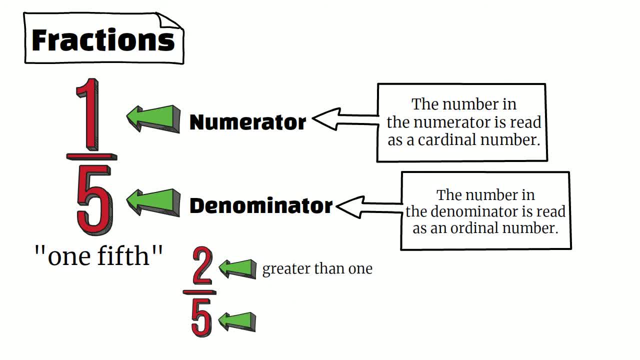 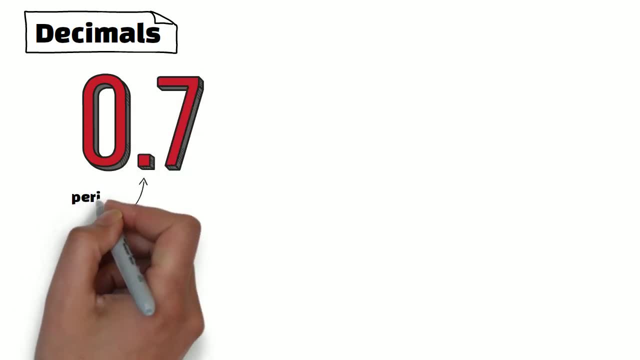 is greater than one, then we add S to the ordinal number in the denominator, For example two fifths. Let's now move on to decimals. The dot in the middle is the period or the decimal point. This is how we read it: Zero point seven. Or we could read it as we read: fractions: Seven tenths. 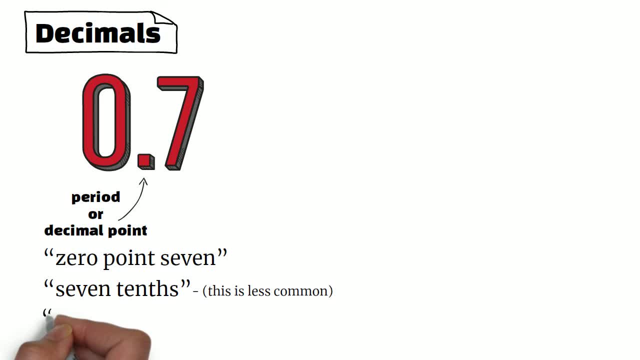 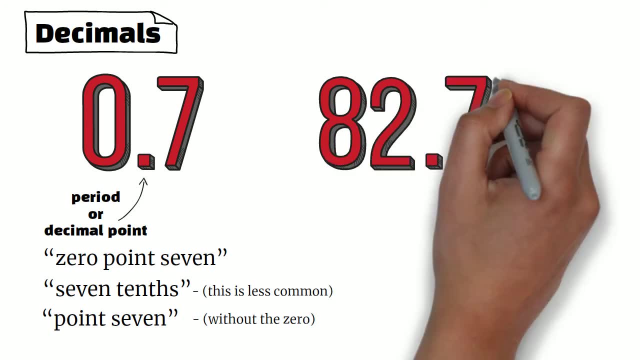 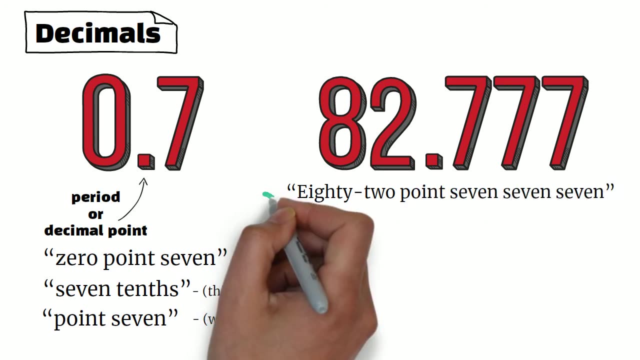 Although this is less common. Sometimes the zero is omitted and we say point seven. If the decimal number is longer like this, then we say eighty-two point seven, seven, seven. We say eighty-two point seven hundred and seventy-seven. This would be incorrect. 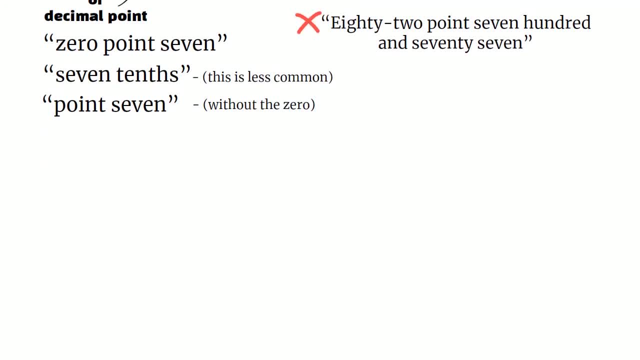 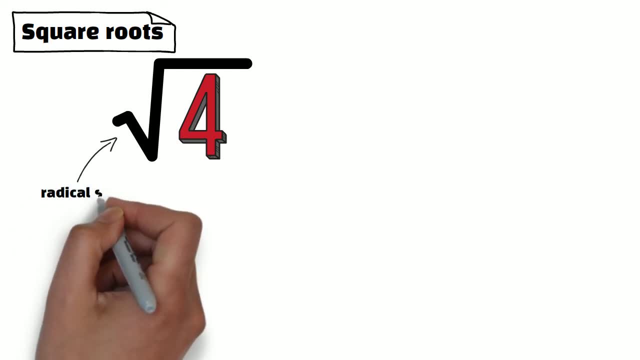 All right, Let's move on to square roots. The first symbol you see is the radical sign. Sometimes it's also called the square root sign. This is how we read this: The square root of four, If there is a number above the radical. 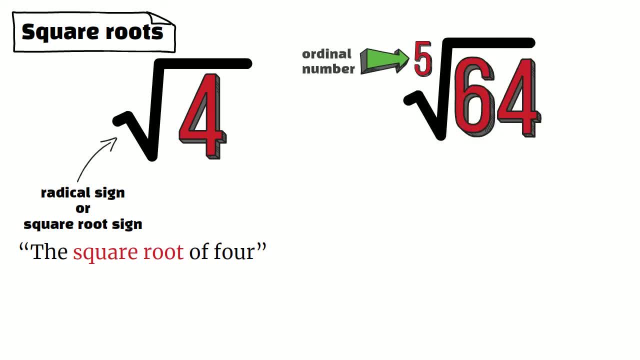 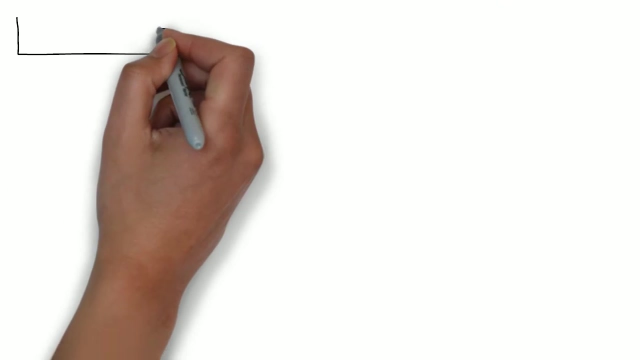 sign, then we use an ordinal number to refer to it: the fifth root of 64.. However, there is an exception: If the number above the radical sign is 3,, then we do not say the third root of 8, but rather the cube root of 8.. Okay, let's now move. 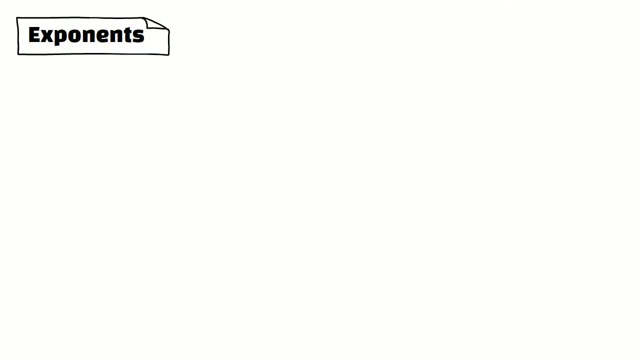 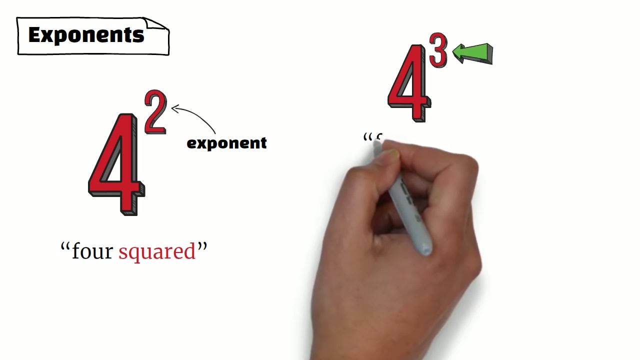 on to the last subsection exponents. The small value is called the exponent. We read the number as 4 squared. If the exponent value is 3,, like in this example, then we say 4 cubed. If the exponent value is greater than 3,, like in this: 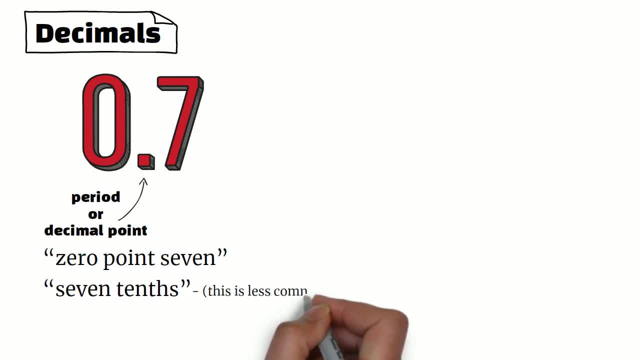 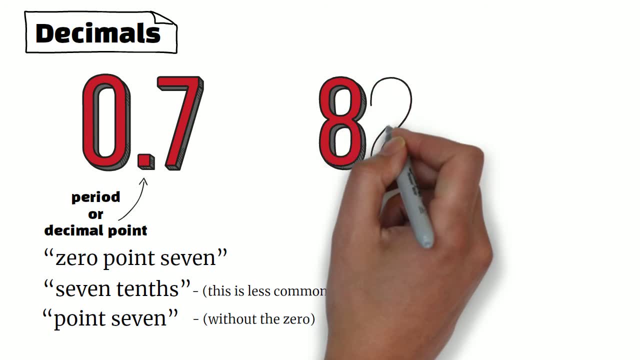 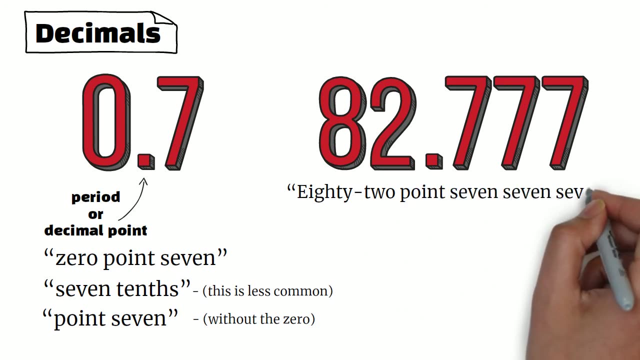 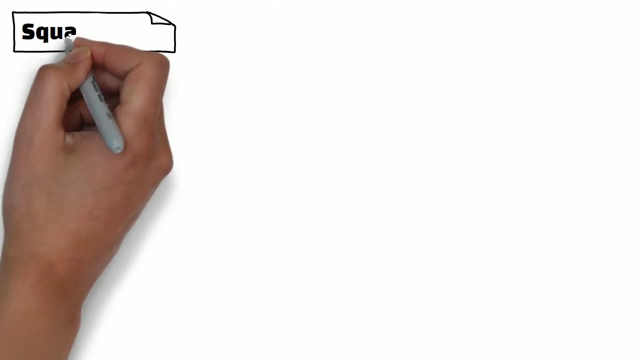 Seven tenths, Although this is less common. Sometimes the zero is omitted and we say point seven. If the decimal number is longer, like this, then we say eighty-two, point seven, seven, seven. This would be incorrect. Alright, let's move on to square roots. 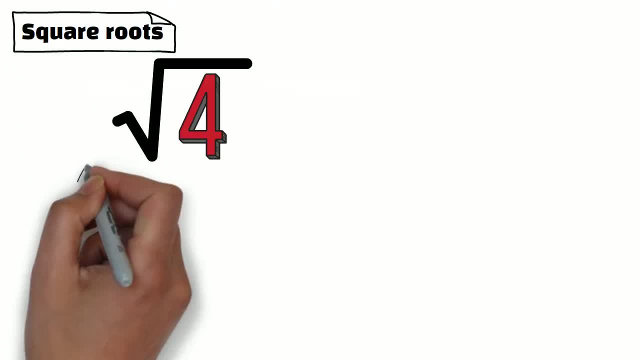 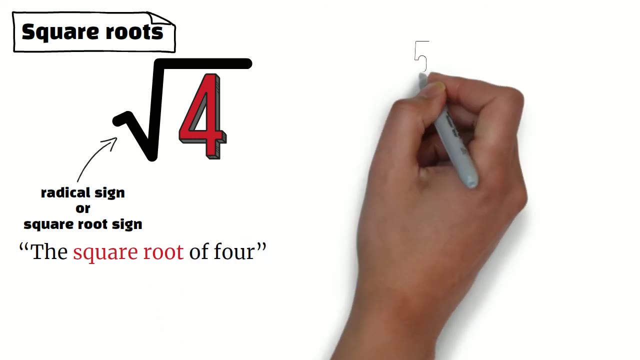 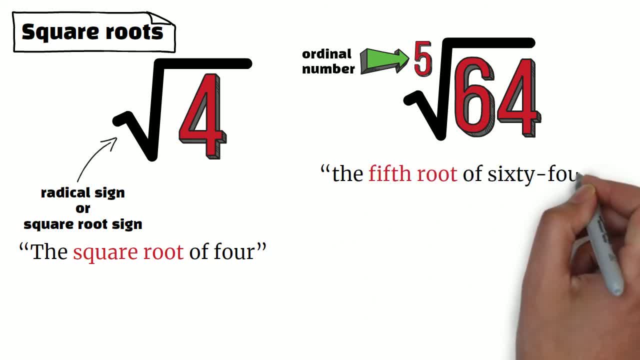